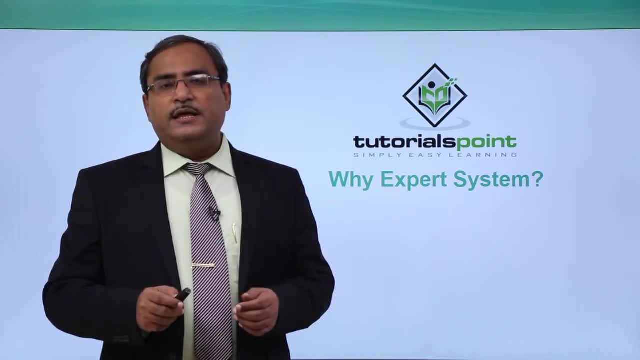 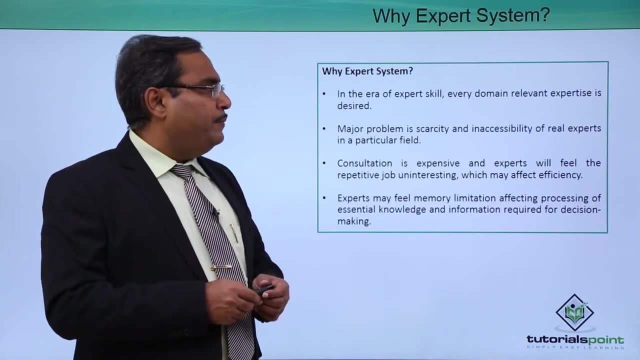 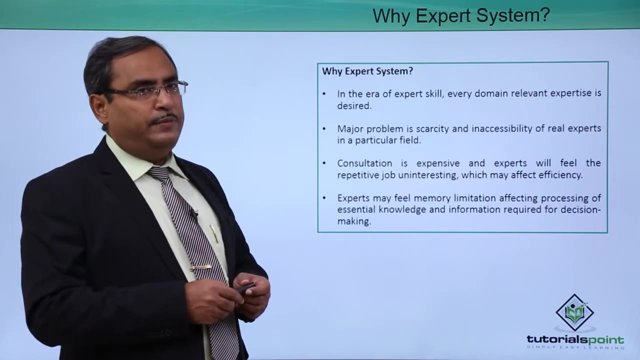 Why expert system? That is a very vital question and we shall search the answers against it. In the era of expert skill, every domain relevant expertise is desired. Major problem is scarcity and inaccessibility of real experts in a particular field. So that is one of the major problems. 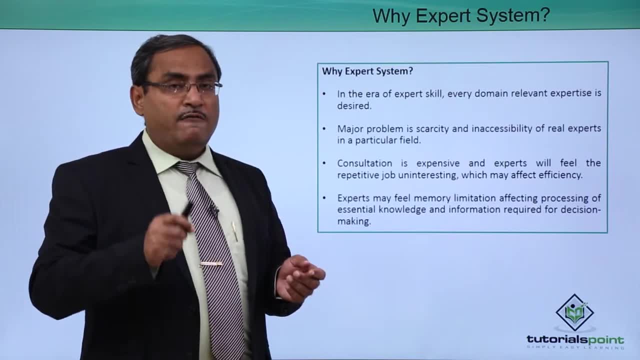 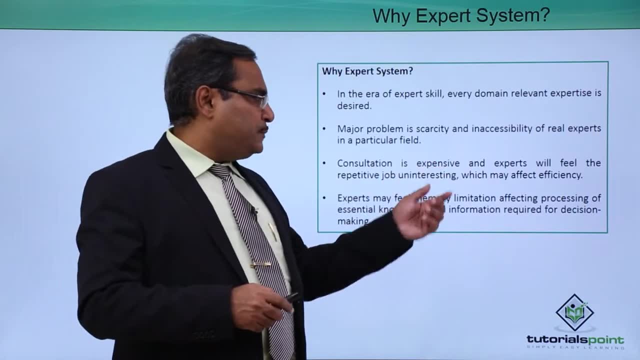 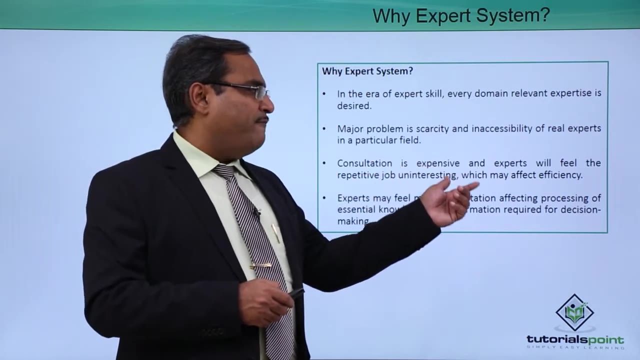 we may face For a particular domain, for a particular field. finding out the exact and appropriate experts is a challenge for us. Consultation is expensive and experts will feel that repetitive jobs are uninteresting, which might affect the efficiency. So whenever an expert 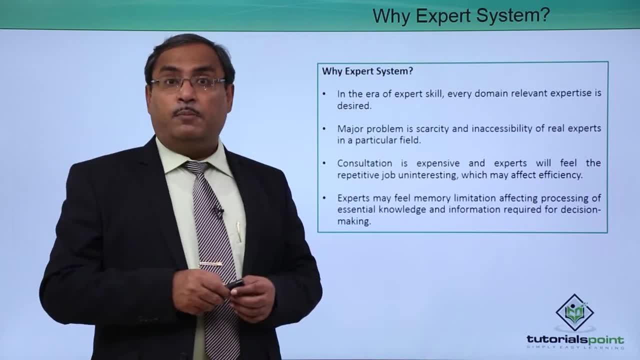 will try to go on doing the same job repeatedly, then monotonicity will be coming. So to get rid of the monotonicity, the prognosis we might face is because there are only the specific conditions that the experts are questioning. they are not capable of finding a solution to. them. The right or the wrong approach will continue for the innovation we proceed. So defining the story of an individual is key, especially the youth in refugees and Тоca Italy, whoкая роли man in Some Indian country where they may40s very 11 years of age. 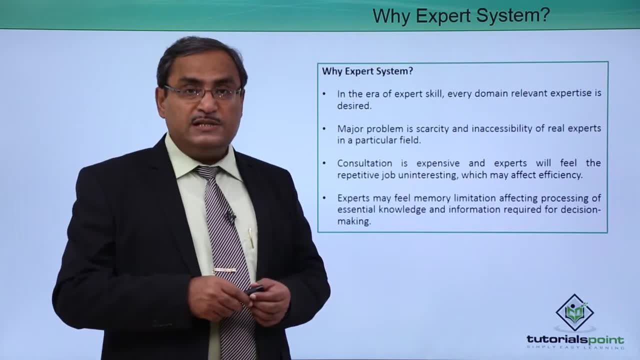 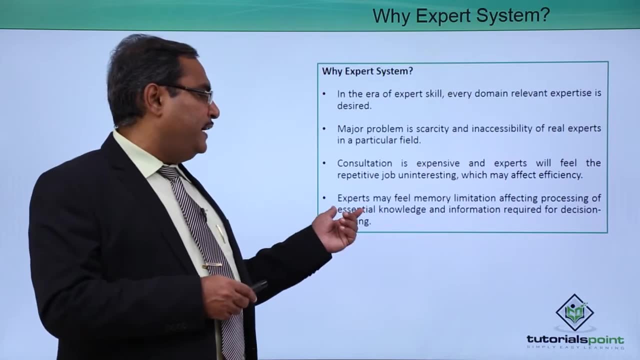 peso a street battle against badар nyar s organiza erfasiastuness sm. meanwhile, ele rewarded in επιt caused by an job will become monotonous to the respective experts, So the performance may get degraded. Experts may feel memory limitation affecting processing of essential knowledge and information. 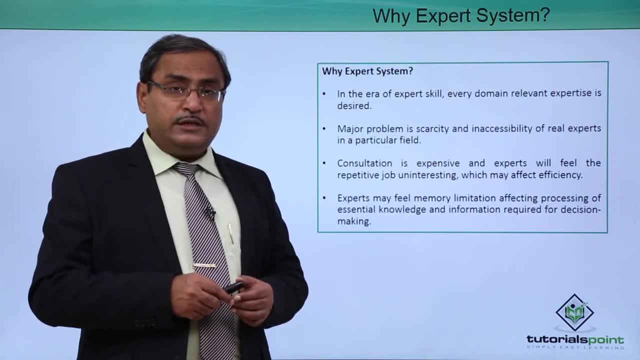 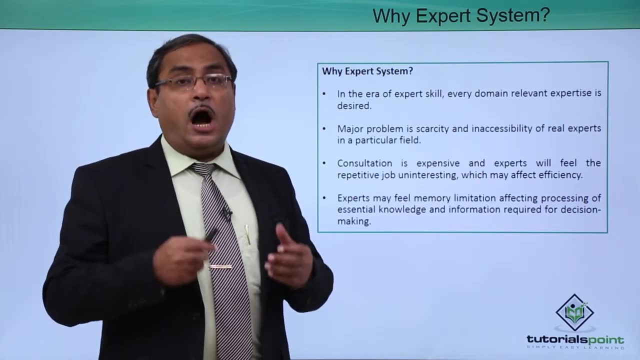 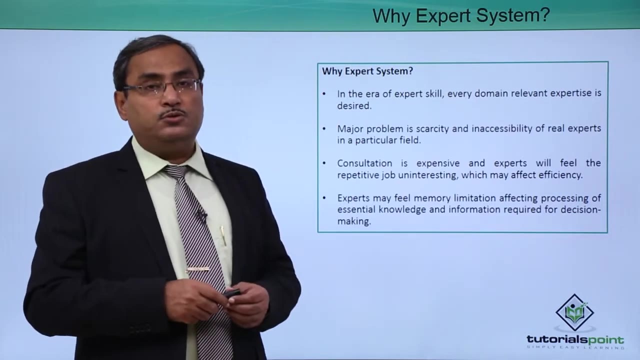 required for decision making. So obviously, the decision which will be made by the expert will depend upon his or her memory capacity, how much he or she is knowledgeable. So that is why the decision will be varying from one expert to another. expert Researchers and developments in 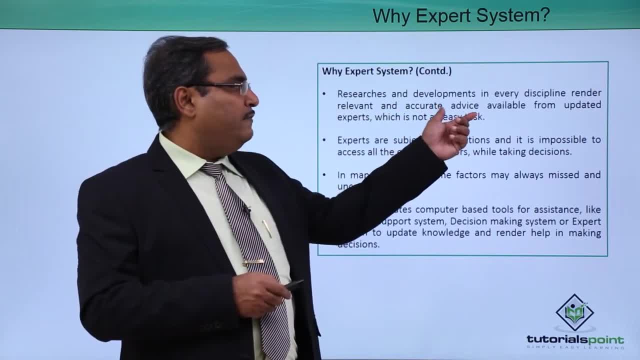 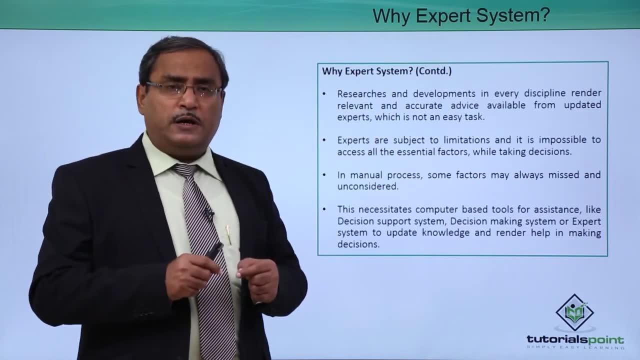 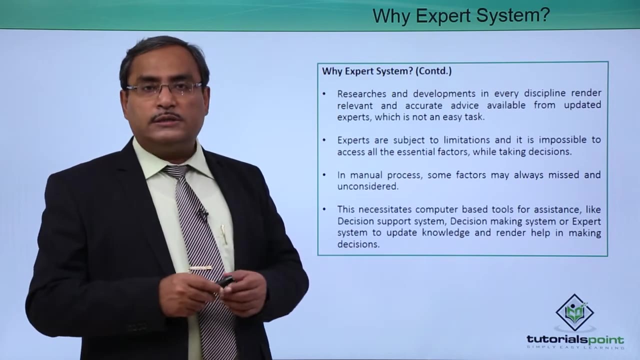 every discipline render relevant and accurate advice available from updated experts, which is not an easy task. So finding expert in the respective domain and getting this expert deployed into the particular domain and problem is always a big challenge for us. Experts are subject to a lot of challenges. They are subject to a lot of challenges. They are subject to a lot. 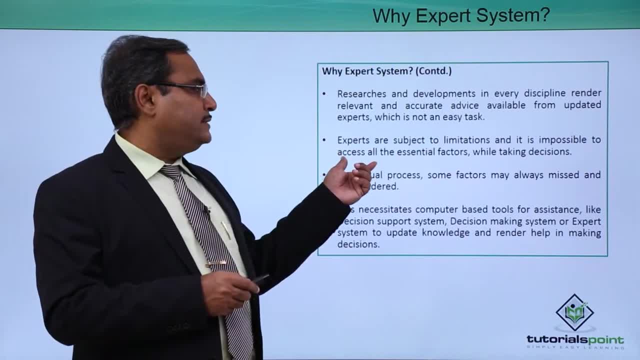